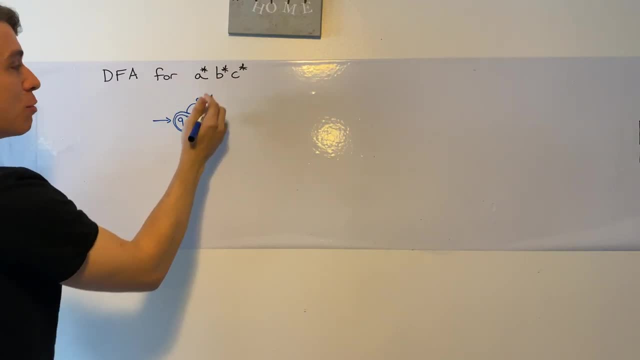 But suppose now? well, suppose that next we have a B. Well again. well, we can't stay in this state, because if I did something like this and I stayed in the same state, well, if I take the B transition. 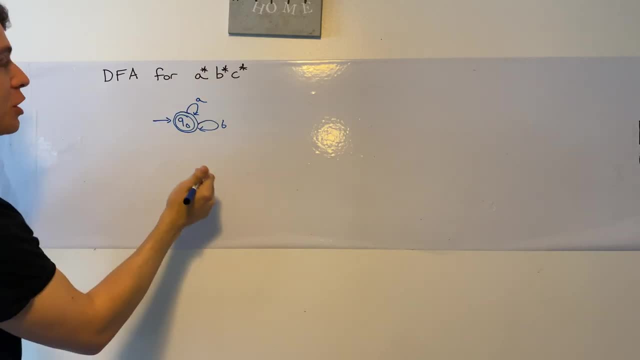 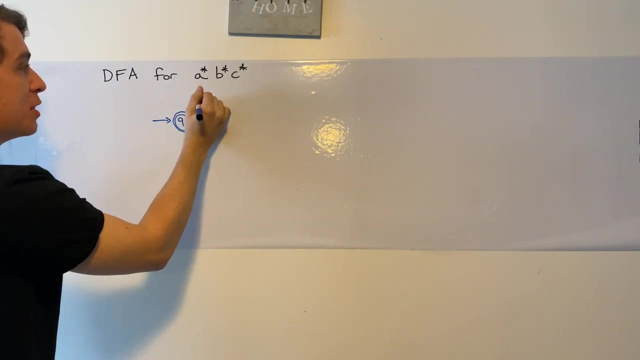 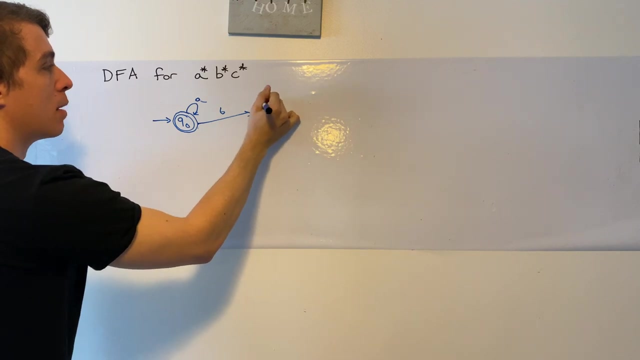 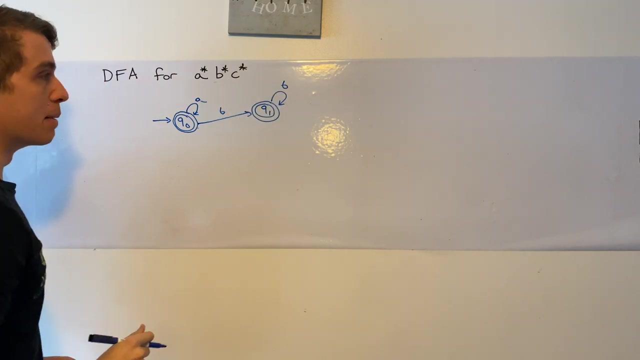 then I'm allowed to take the A transition, And so I would have a BA in the string, and that's not allowed according to this. So let's go to a different state. So I'm going to have a state here Q1, and I can have any number of B's here, So let's just be allowed to read any number of B's. 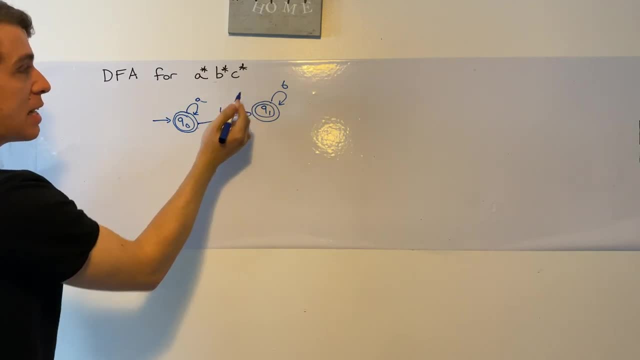 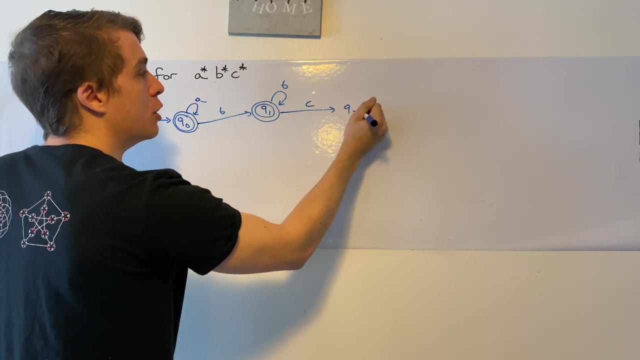 And, like we did before, we can have any number of C's after. but suppose that there is a C, So then let's read the C and go to a state Q2. And we can read any number of C's there, just like the other cases. 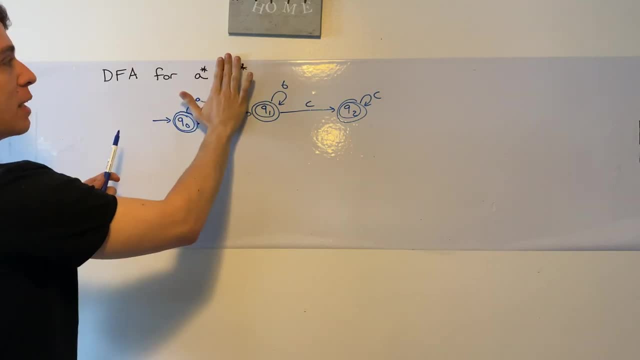 But suppose that there are no B's in the string. So if there are no B's in the string, then we have A's followed by C's, which is perfectly allowed. So if we have a C from Q0, then we should be able. 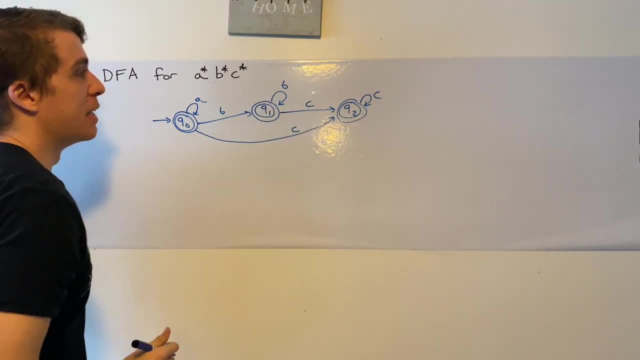 to read as many C's as we want right after those A's. But here are the other cases. So what could happen? Well, if we have a C from Q0, then we should be able to read as many C's as we want. 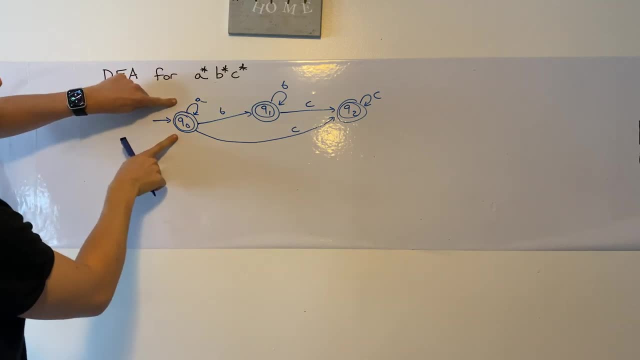 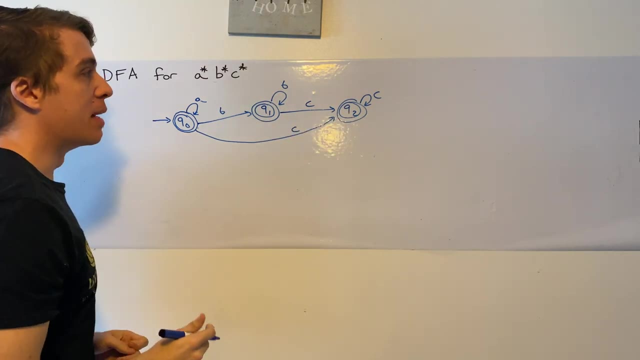 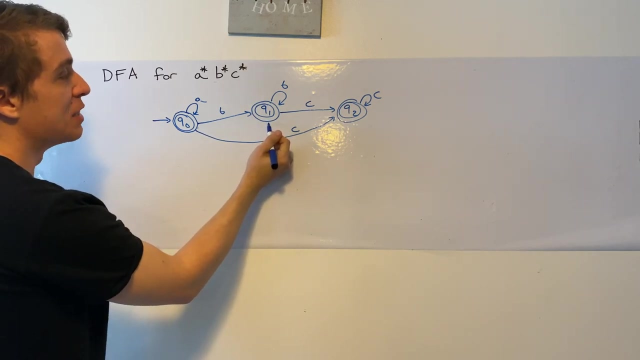 Well, the alphabet here is ABC, So the Q0 state has an A, B and C, so that's fine. The Q1 state has only a B and a C right now and it's missing an A transition, So let's think about what that means. So if Q1 has an A, if we're in Q1 and we're destined to- 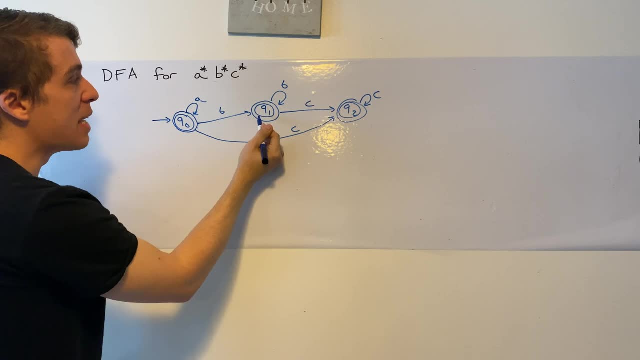 read an A, that means we've read at least one B. But then if we read an A, well, this is not allowed by the language that we're destined to read. So if we read an A, then we're destined to read an A. 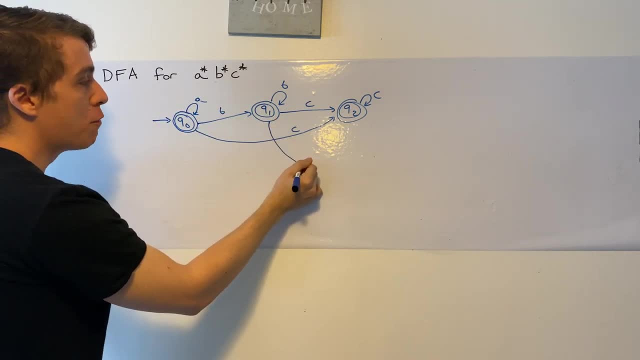 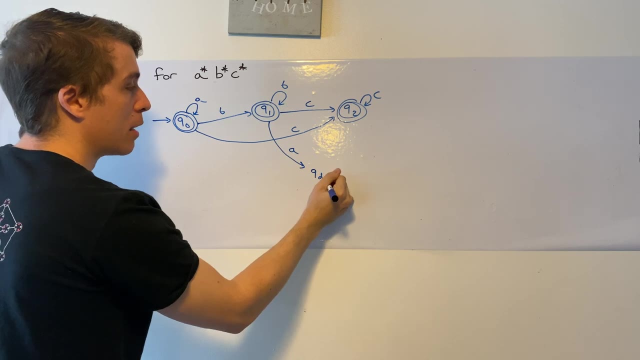 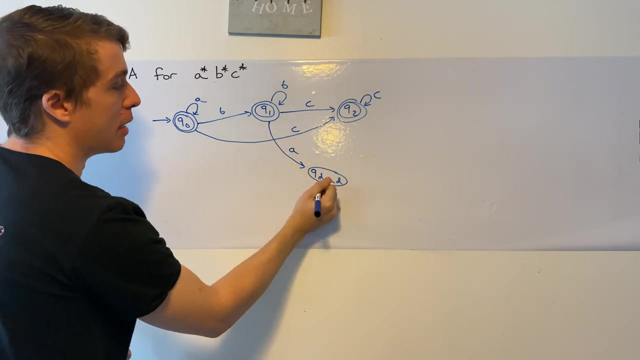 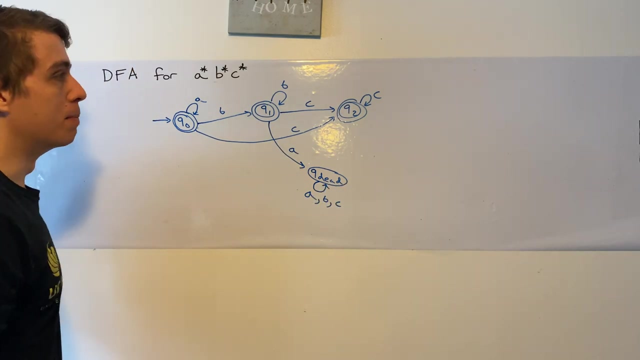 So that means if we read an A at this point we should not accept. So I'm going to have a state here called Qdead because it's called a dead state And once we're there we should never accept the string, which means here that I'm going to self-loop on all possible inputs.